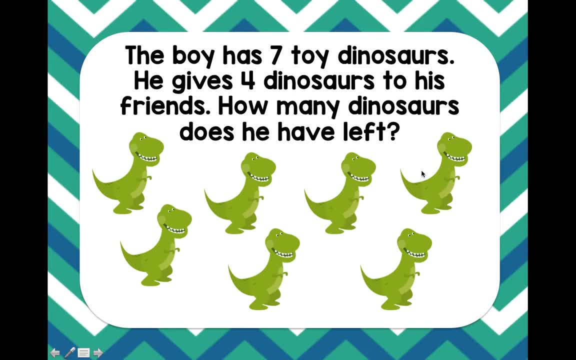 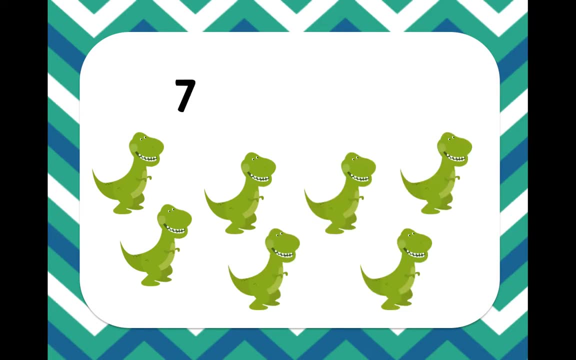 how many dinosaurs away? Four, So let's take away four. One, two, three, four dinosaurs away, And how many dinosaurs does he have left? Count them Three. Good job. So he has seven dinosaurs minus four dinosaurs One. 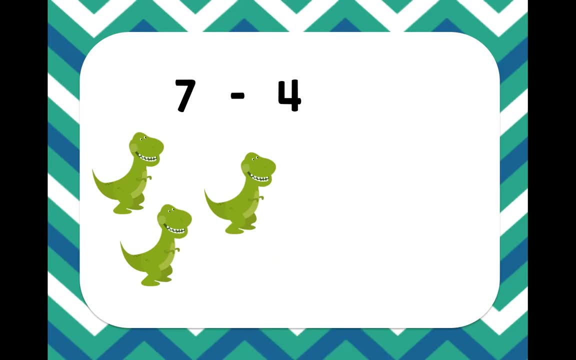 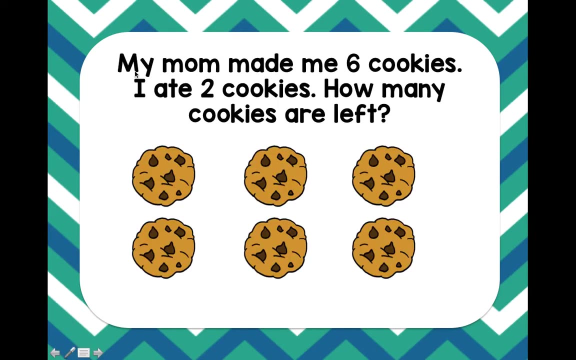 two, three, four dinosaurs equals three. Good job, All right, let's read the story. Let's read this one. My mom made me six cookies. I ate two cookies. How many cookies are left? So how many did she make me Six? And how many did I eat Two? So how many do we take away? 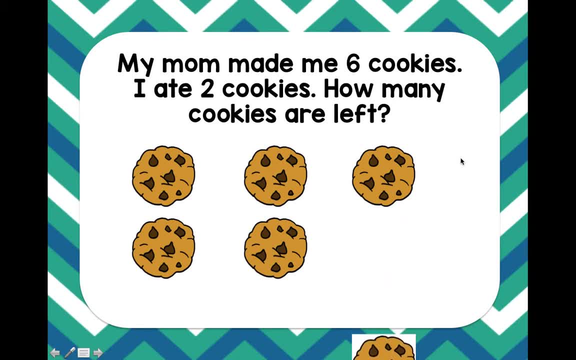 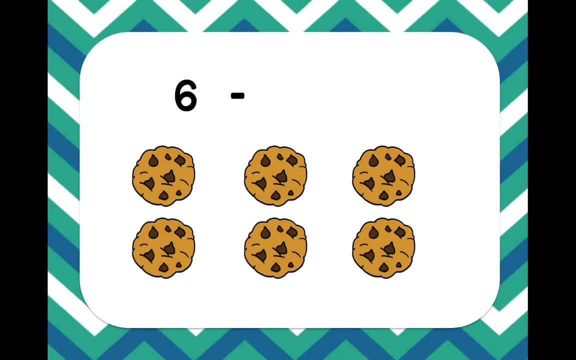 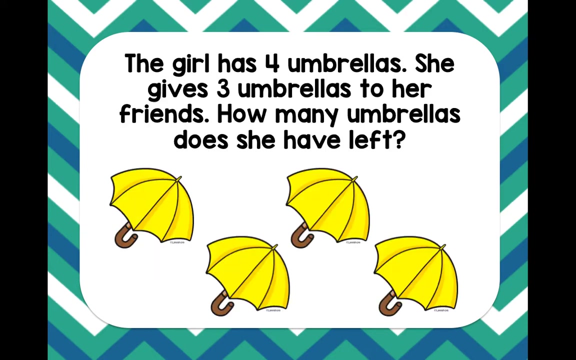 Two cookies, One, two. How many cookies? Four Good. So if I have six minus how many cookies, did we take away Two. How many did that equal? Do you remember? Take away two, One, two, It equals four Good. And our last: 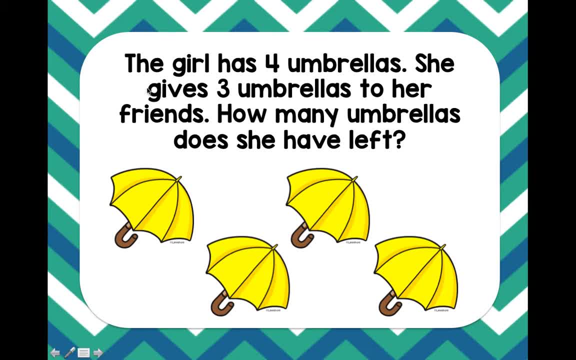 story. Oh, nope, Just kidding, I have two more story problems. The boy has seven dinosaurs. The girl has four umbrellas. She gives three umbrellas to her friends. How many umbrellas does she have left? How many umbrellas does the girl have? Four, One, two, three, four, And how many? 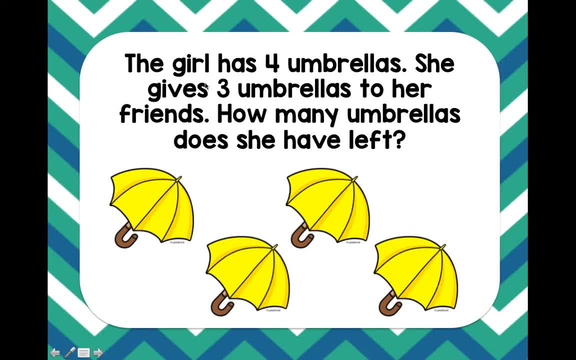 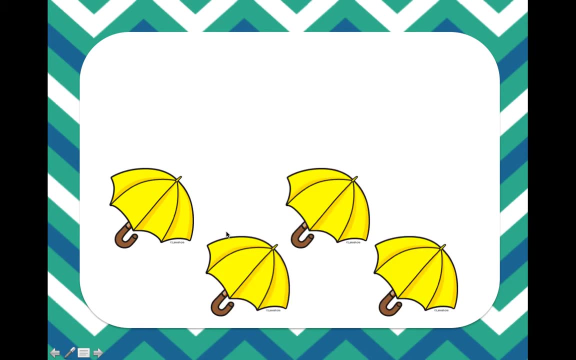 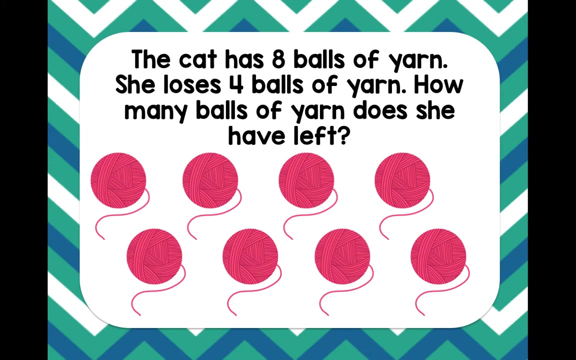 umbrellas does she give away Three? She gives three umbrellas to her friends, So we take away three. One, two, three. How many umbrellas does she have left? One Good. So if we write the equation, we write: four minus three. One, two, three equals how many One Good. All right, The cat has eight. 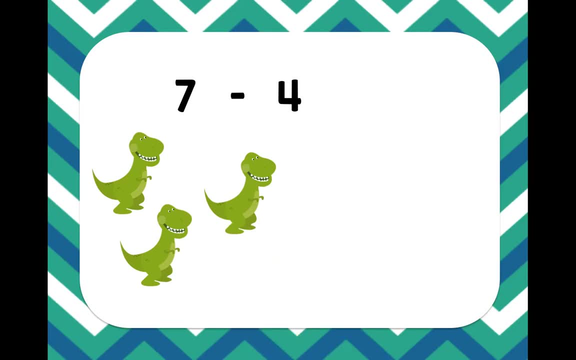 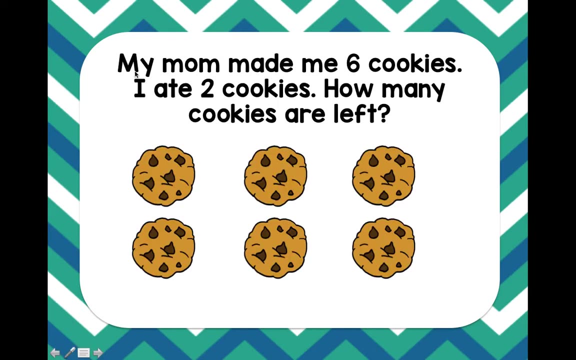 two, three, four dinosaurs equals three. Good job, All right, let's read the story. This one: My mom made me six cookies. I ate two cookies. How many cookies are left? So how many did she make me? Six? And how many did I eat Two? So how many do we take away? Two cookies? One? 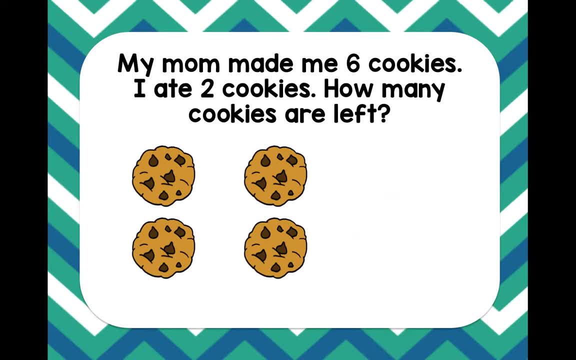 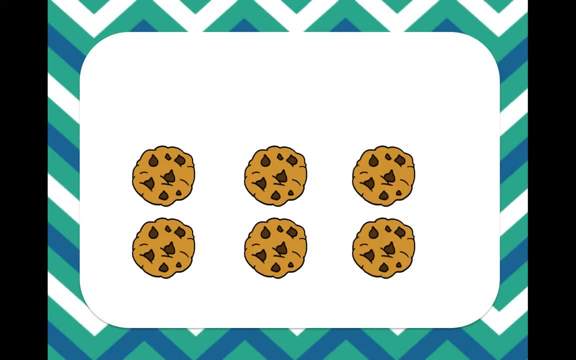 two. How many cookies Are left? Four Good. So if I have six minus how many cookies, did we take away Two. How many did that equal? Do you remember? Take away two, One, two, it equals four Good. And our last story: 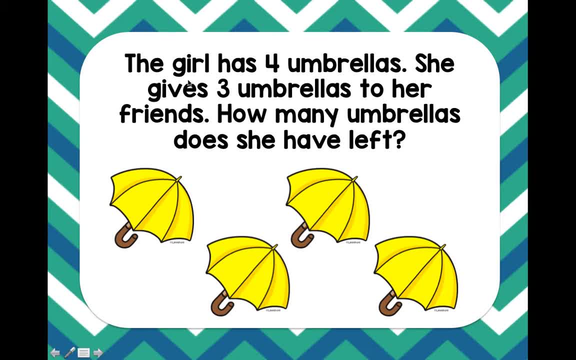 oh, nope, just kidding. I have two more story problems. The girl has four umbrellas. She gives three umbrellas to her friends. How many umbrellas does she have left? How many umbrellas does the girl have? Four, One, two, three, four, And how many? 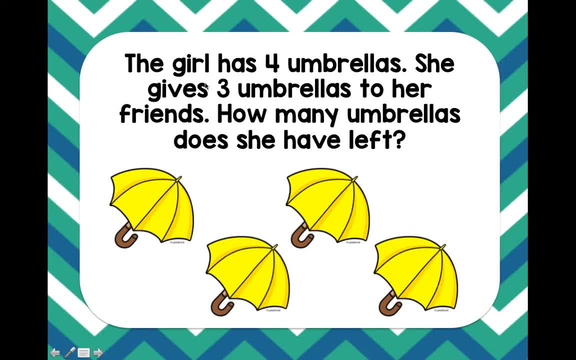 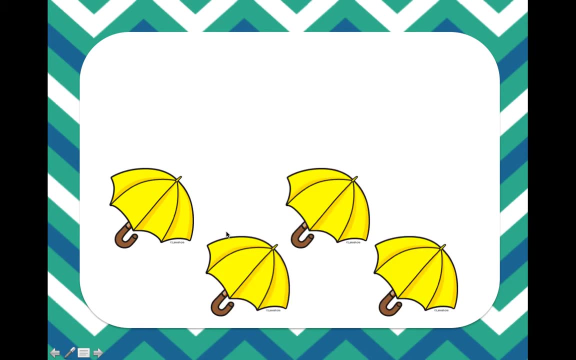 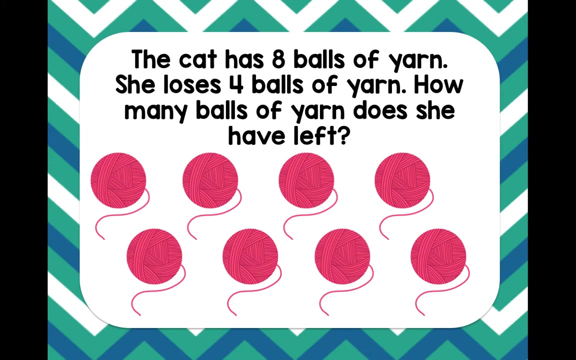 umbrellas does she give away Three? She gives three umbrellas to her friends, So we take away three. One, two, three. How many umbrellas does she have left? One Good. So if we write the equation, we write four minus three. one, two, three equals how many? One Good. All right, The cat has eight. 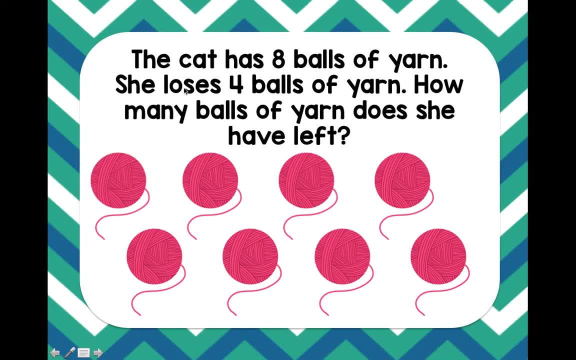 balls. Four balls of yarn. She loses four balls of yarn. How many balls of yarn does she have left? So the cat has how many balls of yarn? Eight, One, two, three, four, five, six, seven, eight balls of.